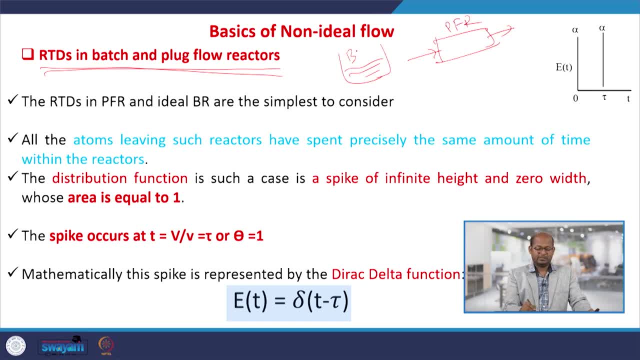 in the batch reactors we usually conduct when experiments. So we just take the reactors and put the reactant mixtures inside of the reactors and we spend for 30 minutes, 20 minutes. once the reaction is over, then we take out all the reacting mixtures or the product mixtures. 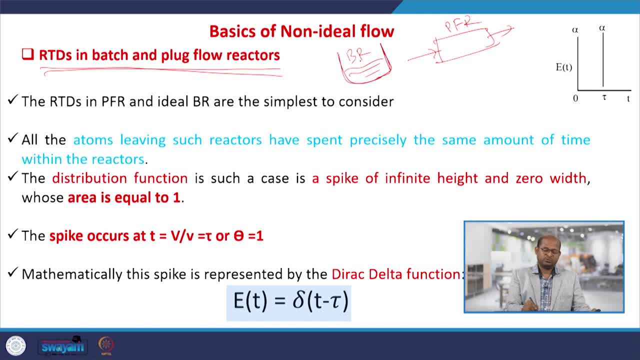 So here in this batch reactor, there is no inlet, no outlet, So this part is no, and this no means inlet, input, output is no, there is no. So therefore, here we can say that this batch reactor is an ideal reactor. So here all the 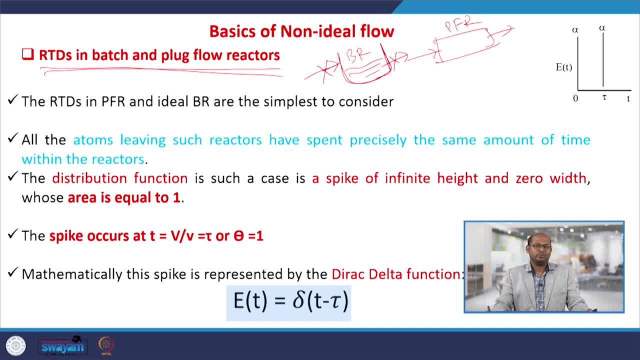 molecules, whatever we charged inside of the reactor, spent equal times for that total experiments In case of the perfectly plug 4 reactors. also, if we say that this is the reactant molecules, so once it is entered inside of the reactor, after that it gradually moves this way. So 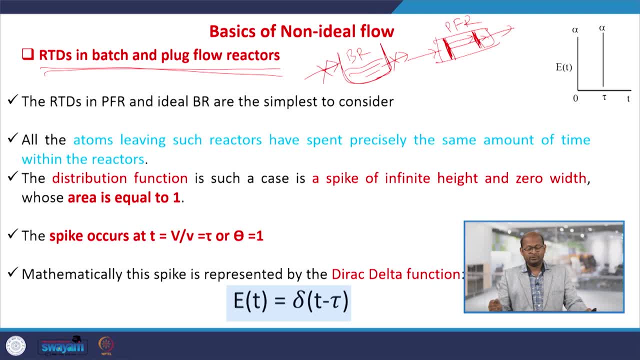 the moments of that reactant molecules spending equal time. So in these two cases we can say: the reactors are ideal. So in this case, when the reactor is ideal reactor, so here you can see that the E t curve, E t means residence time- distribution functions for: 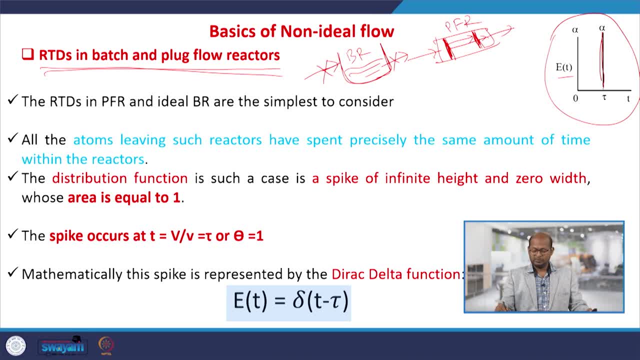 this type of reactors usually a vertical lines is coming, So that is called spike. This is called spike 1 Reactors, when batch reactors or plug 4 reactors. if we conduct the tracer test in this type of reactors, these are- since these are the reactors are perfect, ideal reactors. So then, 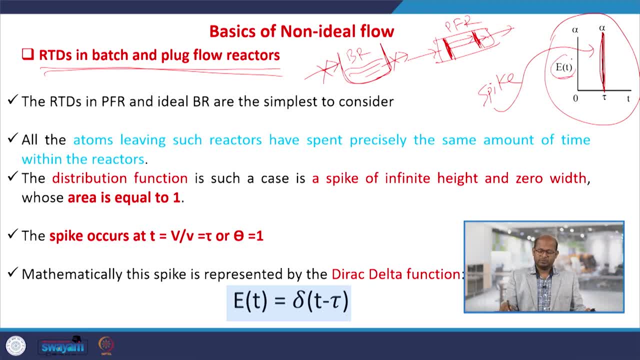 if we want to find out the E t means, first we have to find out the C curves for this particular reactors, Once we know that concentration at a particular time, and then we convert that into residence time distribution functions or E t 2. E t curves, that is, means at this particular time. that is the tau. it would be spike. So 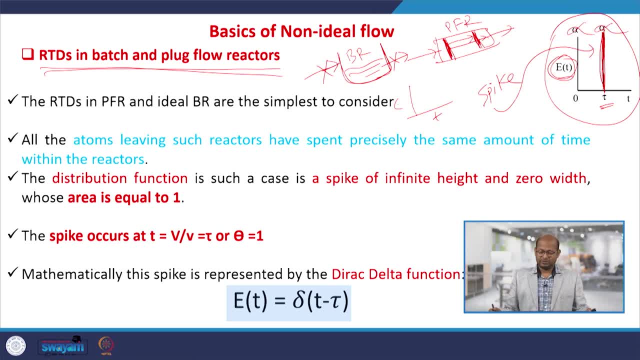 with infinite height. So therefore, this type of means when ideal reactor is theirs. this is nature of ideal, natures of E curves. In most of the cases, E curves usually comes like this, but when it is ideals, 3.5.. 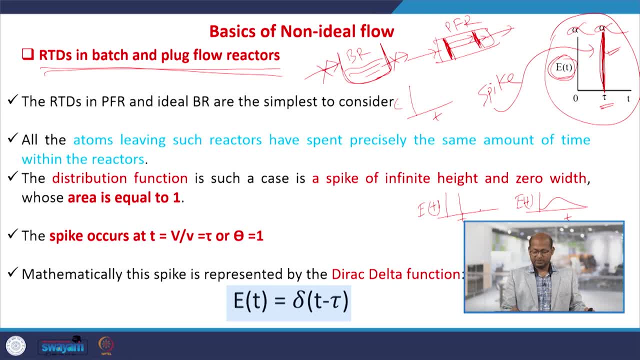 It would be like this. Sometimes it is coming like this, So it may be like this. So it indicates ideal to non-ideal natures of. that means from the E curves we can say whether the reactor is perfectly ideals or not. 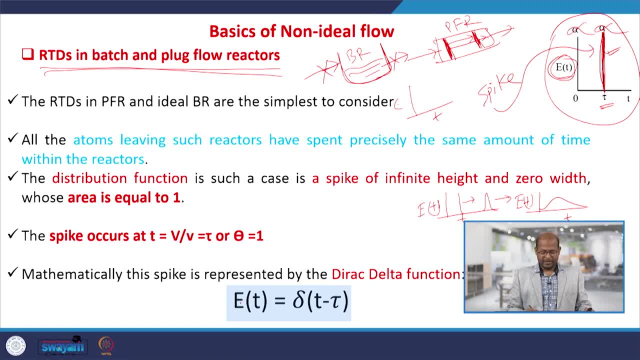 4.. So now this type of spike, or E curves. mathematically, this spike is represented by direct delta functions and it is expressed in terms of E. t equals to delta t minus tau. So this is what we say. So for batch reactors and PFR reactors: plug flow reactors, ideal batch reactors or ideal. 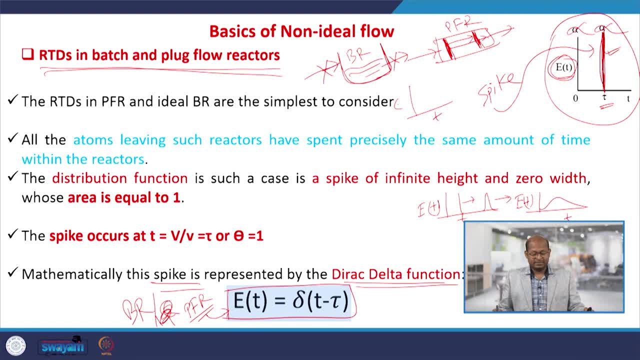 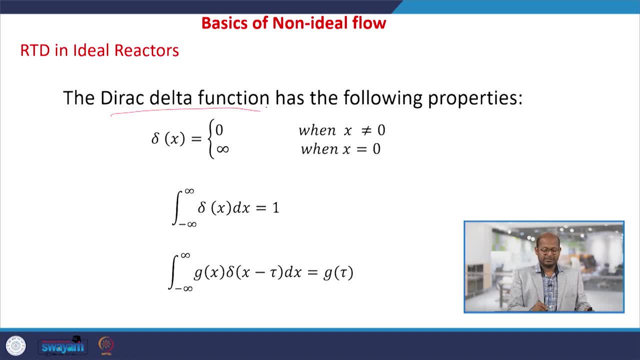 plug flow reactors residence time distribution function. E t is delta t minus tau. So what is direct delta functions? So delta function has the property delta x equals to 0 when x not equals to 0.. 5. And delta x equals to infinite when x equals to 0. 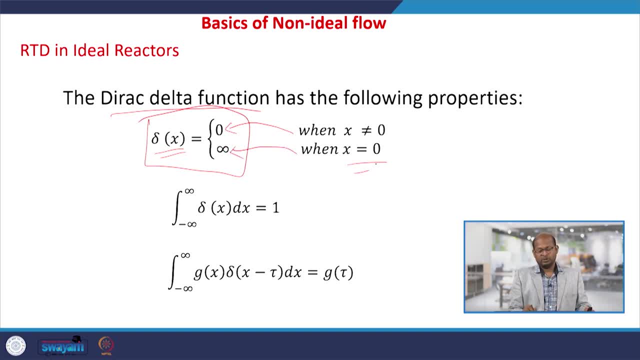 6. So delta x is not equal to 0. 5. So delta x is not equal to 0. 5.. 6. equals to 0. So this is the property of a direct delta functions and delta functions. 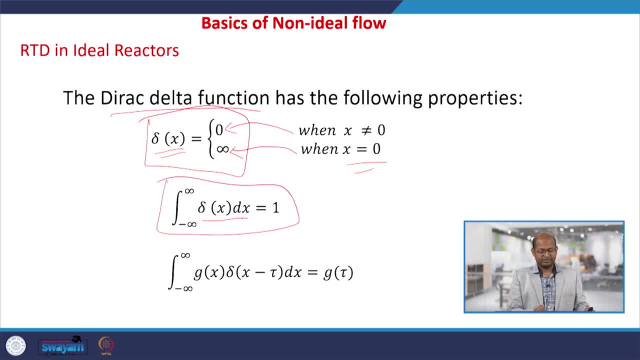 we can express: minus infinite to infinite. delta x, dx equals to 1. if it is like this, integration, so then it would be: final result would be 1.. If it is like this, so then this is the delta functions. this is the function gx. So if 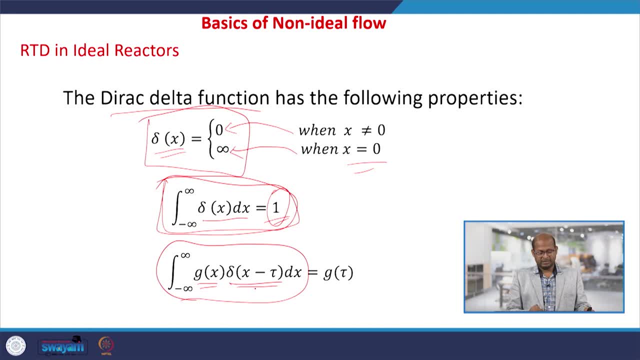 we integrate gx and multiplied with the dx and integrate that with respect to the dx, that result should be g tau. this tau would be here. So this way we can get g tau. that is the results. So this is the delta functions, how we can mathematically express, or its property. 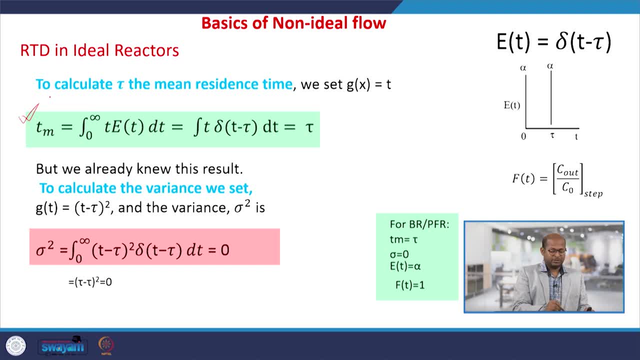 that we have discussed. So now means mean times, mean residence times or Tm. that usually express mathematically this way these expressions. So here we said that this For ideal reactors, ET, Residence-time distribution function, express this way. So this ET we 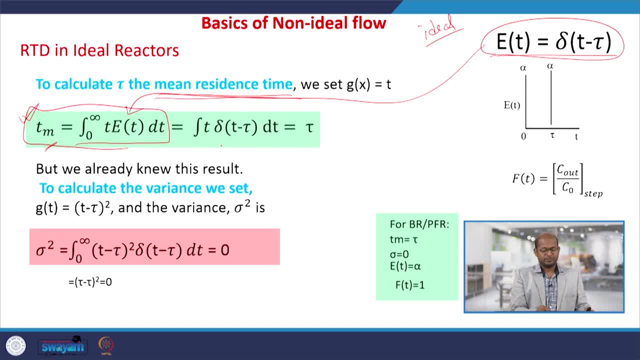 can substitute here. So then Tm equals to T, delta T minus tau, RdT. So the results of this would be tau. so Tm equals to tau mean residence time distribution or mean residence times for ideal reactors. it would be tau. 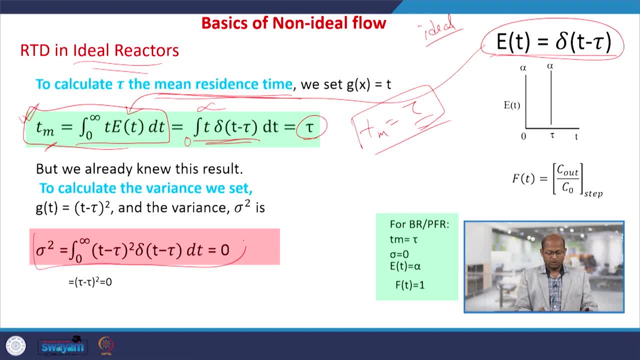 Similarly for variance also. so variance we can express in terms of sigma square 0 to infinite T minus tau, whole square Et DT. this is the variance definitions. So here also for ideal reactors, if we substitute this, then this would be like this sigma: 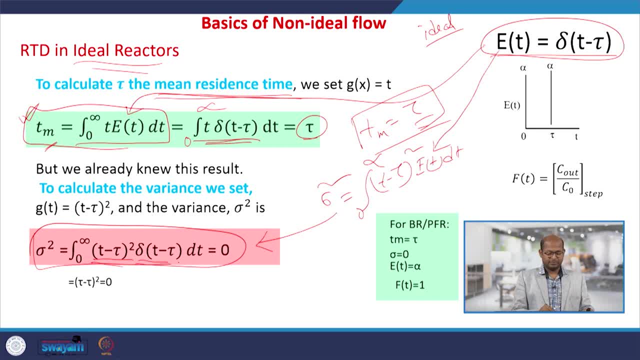 square equals to T minus tau. whole square, delta T minus tau into DT and the result should be: if we integrate this it would be 0.. So here T minus tau, here it would be the tau minus tau square equals to 0. So sigma square equals to 0 for ideal reactors. 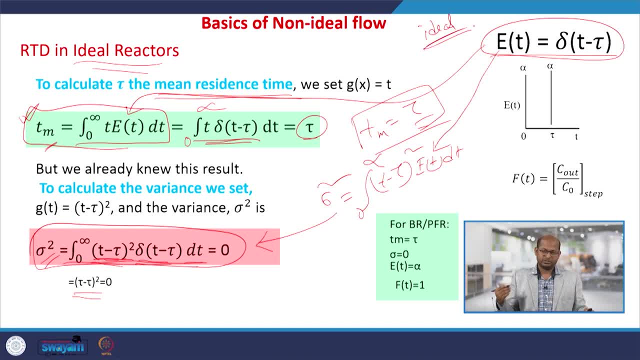 So whenever a ideal batch or plug flow reactors we have the things we can say that for ideal batch or plug flow reactor, mean, time equals to tau sigma. that is, the variance equals to 0 that we have discussed, and Et equals to infinite heights and Ft equals to 1.. 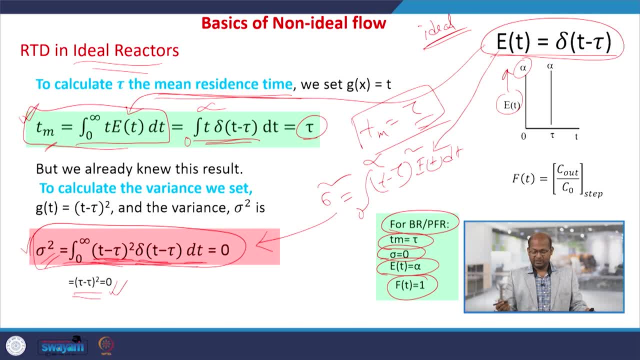 So Ft equals to 1 for perfectly or ideal reactors. here C output that would be equals to 0. So then C0 by C0 equals to 1. we can say that way. So Ft also would be 1 for ideal systems. 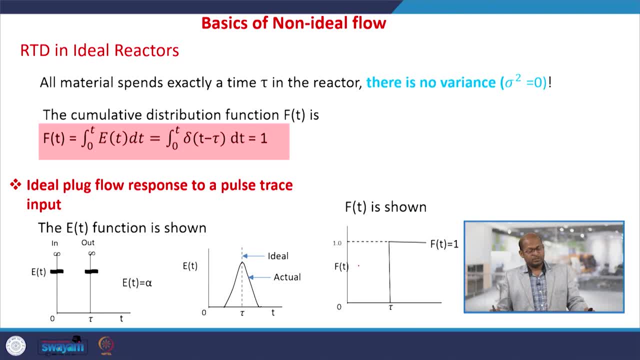 So here Ft also. this way also you can express: So Ft equals to 0 to T Et DT. So here Et equals to delta T minus tau. So here it is substituting here, and then it is 1. you can say So for there is no variance, and Ft equals to 1 for ideal reactor. 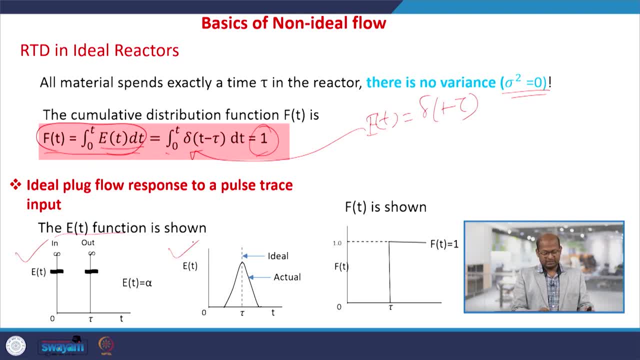 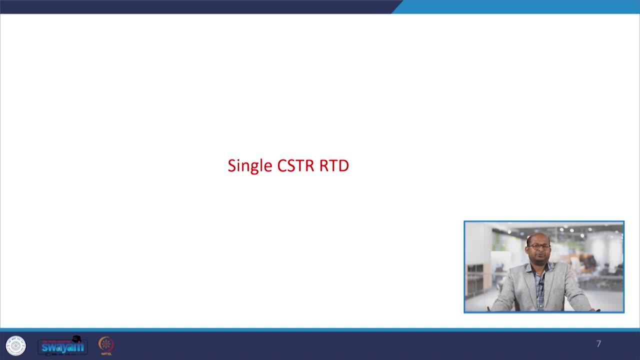 So here E function. So E curves is like that, Et for ideals and actuals is like this, and Ft curves also is like this. that already we have discussed, So no need to discuss more. So now we go for a single CSTR or we have, so means batch reactors and PFRs- ideal plug. 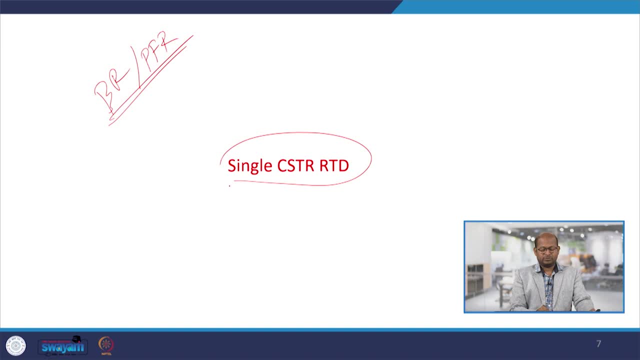 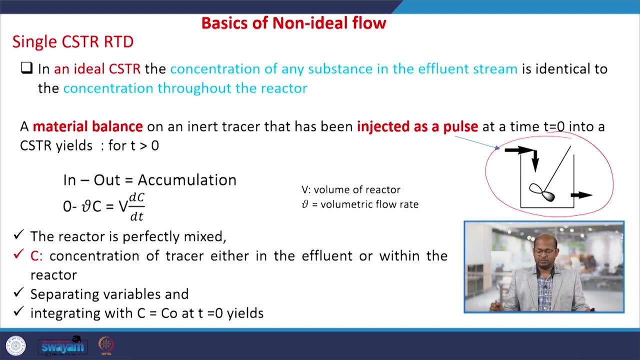 flow reactors and ideal batch reactors we have discussed. Now we are going to discuss for a CSTR reactors, third reactor, that is, the CSTR reactors, and this is called CSTR reactors. So here in this type of reactors mostly means non-ideal natures. usually we found 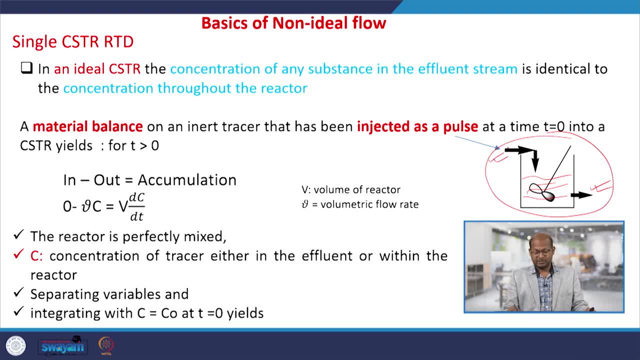 So this is effluent stream concentration here, This is feed concentration, that is, feed entering here and tracer or the effluent after reacting that we are collecting from here and we are analysing. So in this type of reactors, if we do, the material balance on an inert tracer that has been injected. 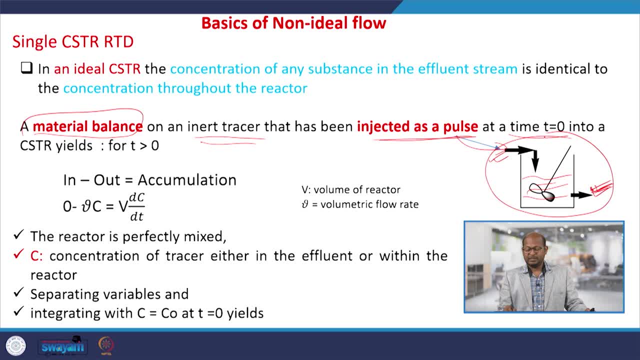 as a pulse. Here we are injecting pulse tracer At a time t equals to 0 and for t greater than equals to 0. So initially just pulse injections of tracers. we have injected here pulse tracer injections. So here outputs from the outlet of the reactors will get the tracers and the time t greater. 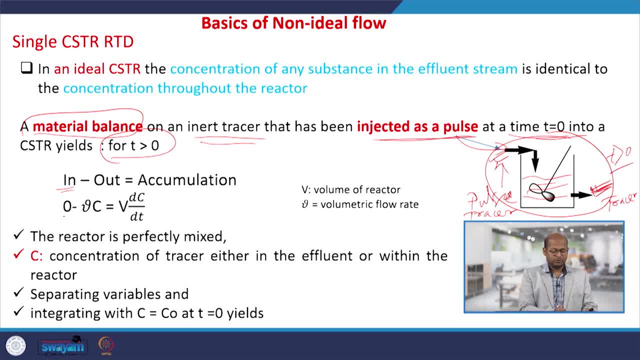 than 0. So input equals to 0.. Since there we have not Once we sort of tracers of treasures that may be 10 millilitre, 5 millilitre, treasure that have been injected here. after that, only feed is passing. there is no treasures. 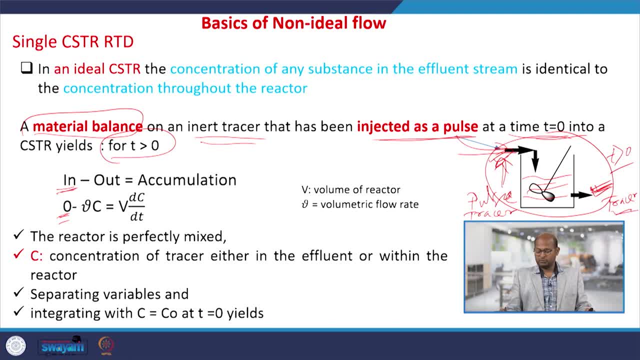 So this input concentration of the treasure is 0 from the output or outlet concentrations. if V equals to volumetric flow rate, is this and concentration at this particular here is C. So this is the concentrations of the treasure that we can find out. and if there 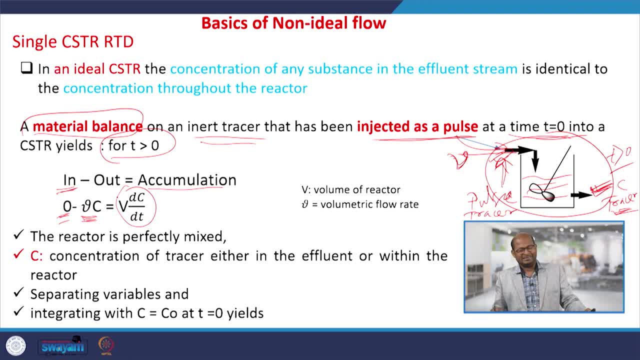 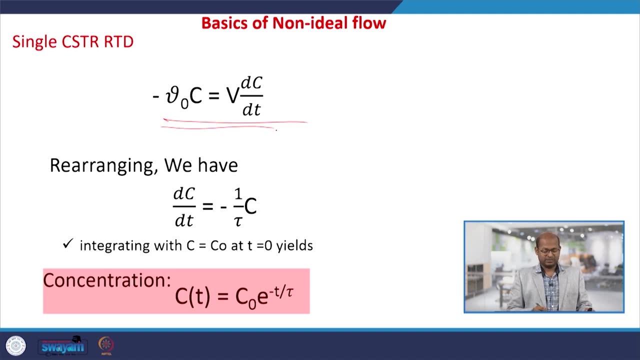 is accumulations inside of the reactor, that we can write V into dC by dt. This way this is the material balance. So here V is the volumetric flow rate and V is the volume of the reactors. So now, if we take these equations and rearrange these equations, so here tau equals to V by 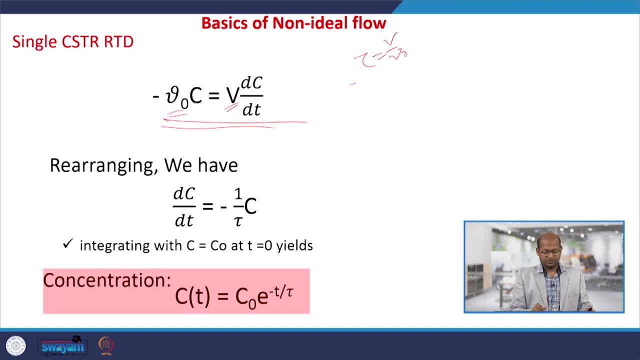 V0.. So here is V, here is V0.. So therefore, tau is coming and rearranging these equations and after that we will find out. So here tau equals to V by V0.. So therefore, tau is coming and rearranging these equations. 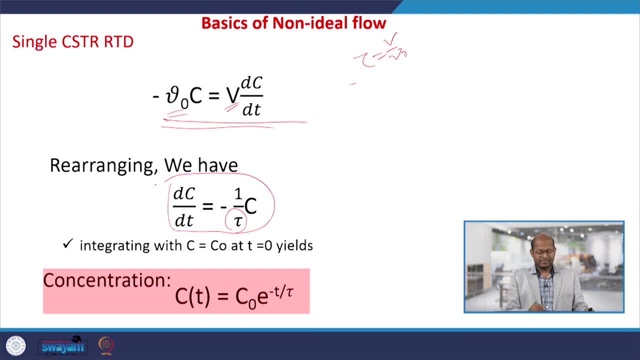 rearranging we can get this. And now we integrate this: differential equations 0 to t, time or tau, dt. Here this equation dC by C minus is also coming. So if we integrate this with respect to this, then we can get the concentrations. So it is wrong, means 1 by tau would be there. 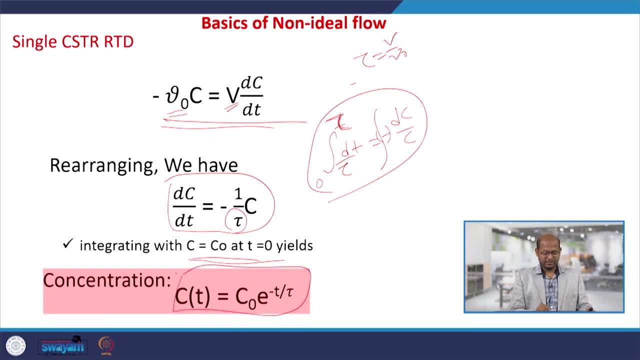 So here after integrating this we can get Ct equals to C0 into e, to the power minus t by tau, The outlet concentrations of the tracer that is coming out from the reactors. here Ct at different times equals to if initial concentration of the tracer that has been. 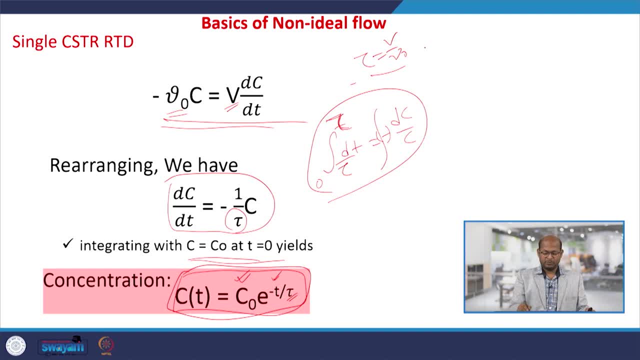 injected at different times times. tau is that fixed volume by volumetric flow rates. So that is the constant. here T is the variable and Ct is the variable. So with T, Ct, rest, tau is known, C0 is known. 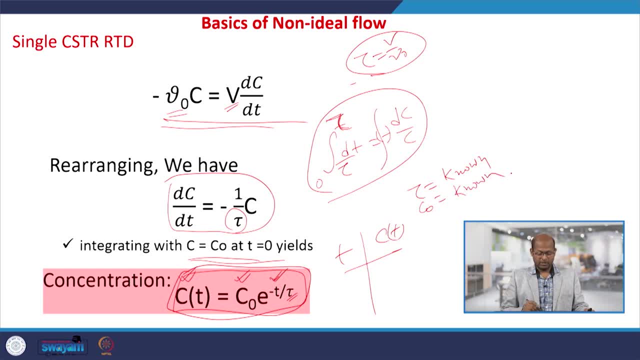 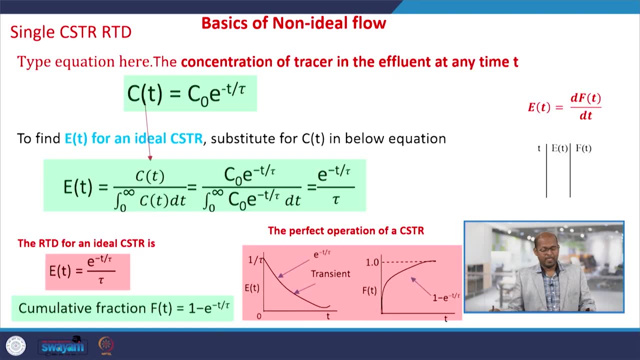 So these are the constant value. So then we can. concentration of the effluent concentrations we can find out. So now for this we have derived from the material balance. So now Et we can express for an ideal, C-H star is equals to this Ct. 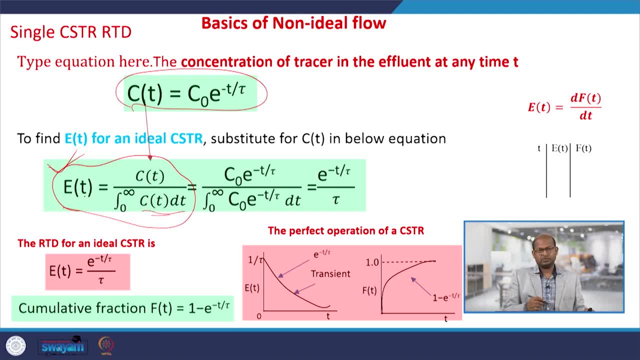 by 0 to infinite Ct, DT, So Et. this way you can write: So now this Ct, we can substitute in hertz and denominator both the places. So then the equation should be like this, and after integrations we can get this: 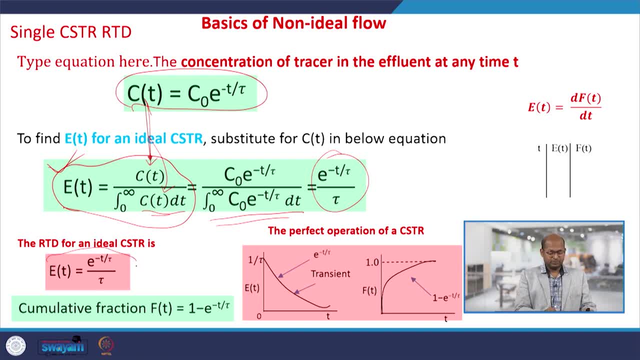 So hertz after Et constant, Sorry. So here now. E equal to Ct by 0 to infinite. So E is equal to cos. E is equal to Ct If curves. we can write this way: E, t equals to e, to the power minus t by tau. by tau that. 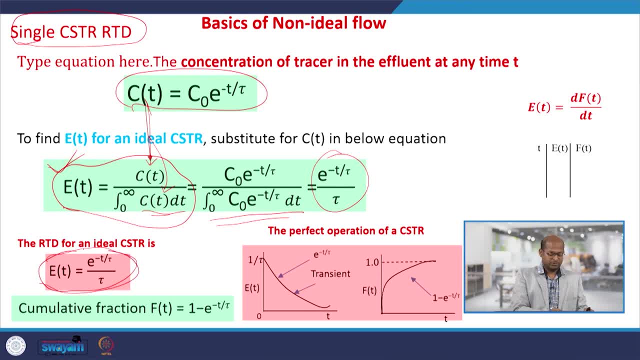 is for single ideal CSTRs. that would be this: Similarly, for cumulative distribution functions, or F t, we can write: F t equals to 1 minus e, to the power minus t by tau. How that is coming that we will discuss So from here. easily we can find out so how that is coming. 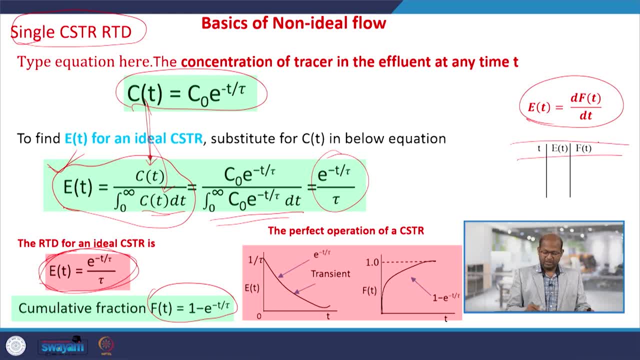 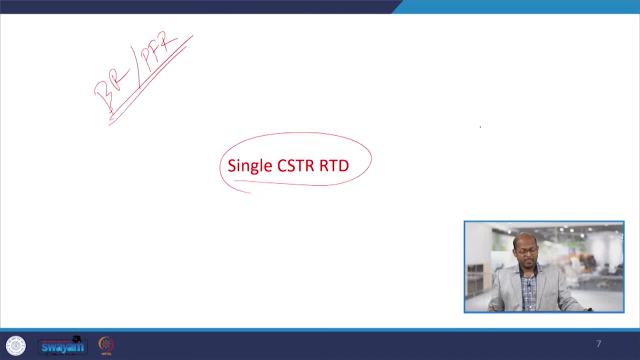 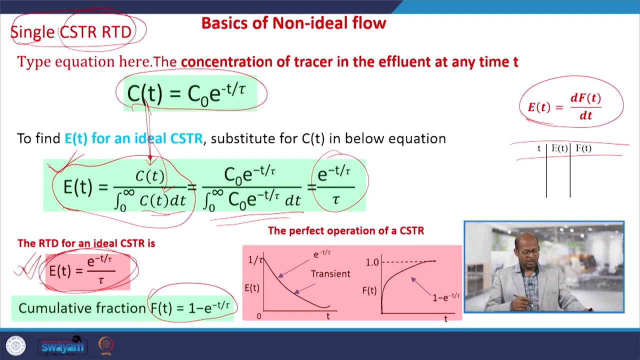 so that we will discuss. So now, if we have these equations, this is E? t. for CSTR reactors, E t. for batch reactors or plug flow reactors, we can express this way, and for CSTR reactors, E? t we can write this way. So this is the basic difference, so you should know about. 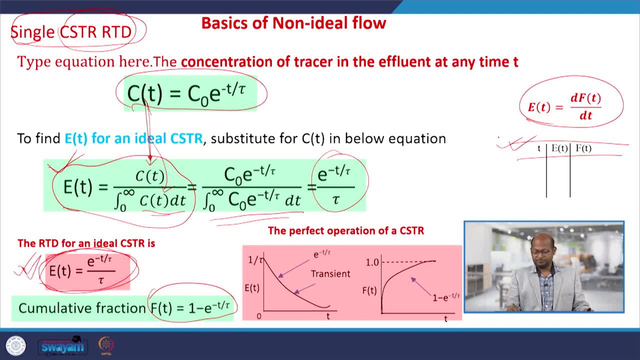 it. So now, if we have this table, So then we can theoretically we can calculate E curves, E t versus t. we can plot F t versus t, we can plot. These are the things known. So then means E t curves would be like this: 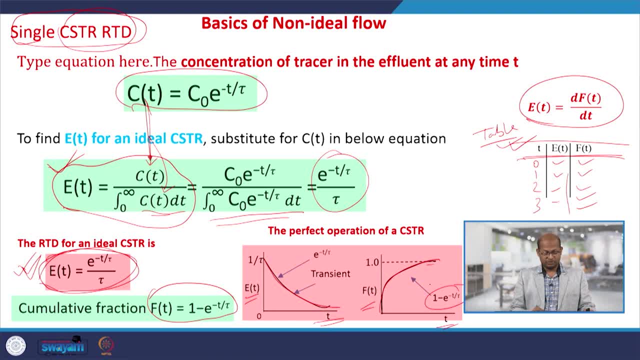 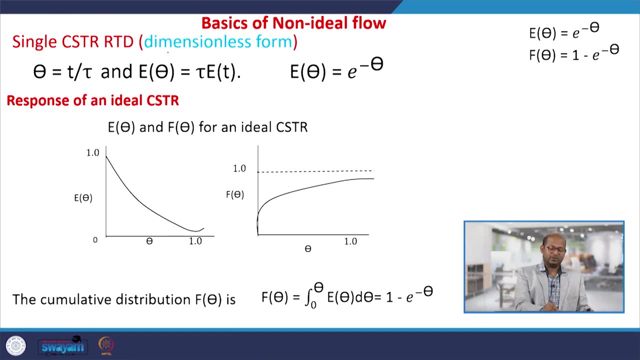 and F? t curves would be like this. So from these equations, and these equations so easily, we can E curves and F? t curves easily draw for the E to the power minus e to the power of is a left. So the fend Ici, the recompense, is going to be like this: So you get d into. 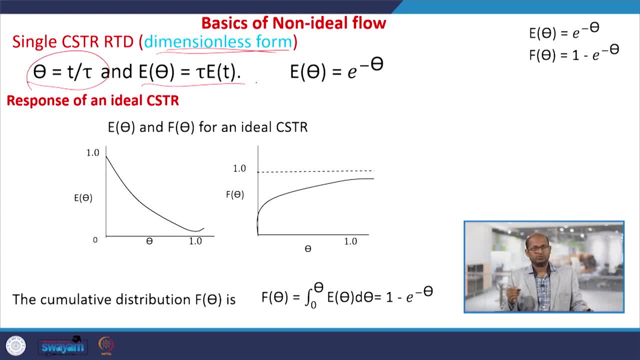 g, which is minus g, which is minus e, to the power minus t divided by L разаaw, applying those exact conditions. So these are the definitions of cost drawing. But in terms of pharmacy, we also have many equations and we have many calculations. we have many equations where f and d are play. 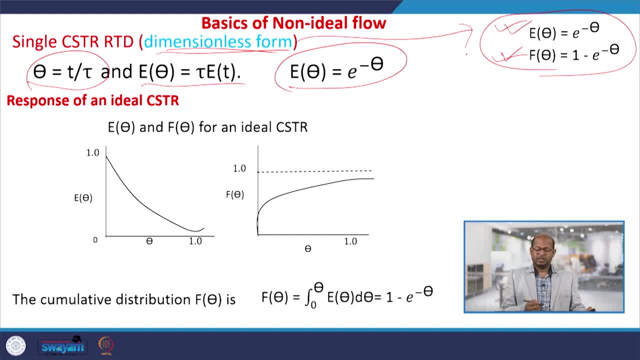 a part, mainly to say like. say, in Europe it is used as a function of disability. In akhirah, the definition of disability symbols and write town and violence is x. Here you can go. the background of this benchmark one. From our paper, you have something like: 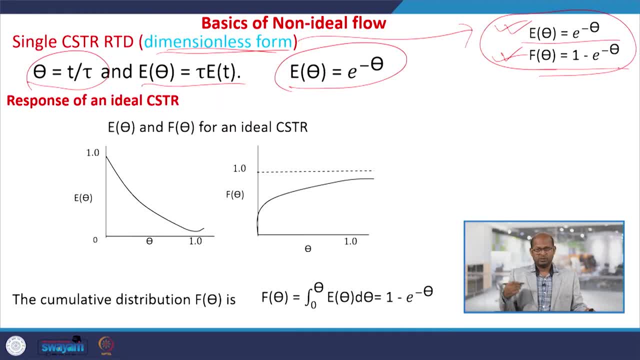 these two dimensionless forms also we can develop. this is E? theta curves, this is F? theta curves. So dimensionless forms, that way also we can express and F? theta. I said how to get it. So here F? theta equals to 0, to theta. E theta, d theta, that would be this. So earlier this, 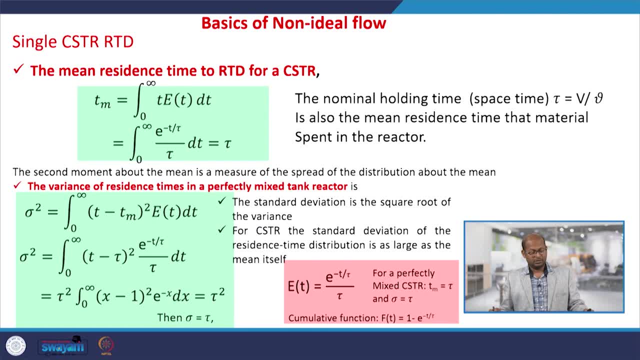 how F? t we got. so this way we can write: Now we are coming to the mean time, mean residence times for a CSTR. So mean residence time, distribution function. or express the equation this way: Tm equals to 0, to infinite TeT, dt. So here Et equals to for a CSTR reactor equals: 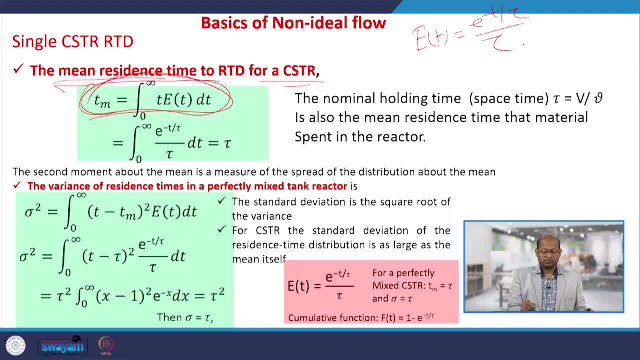 to e, to the minus T, by tau, by tau. So this we are substituting here and then we are doing the integrations Here. one T would be there, I think. So then after integrations Tm equals to tau, So Tm times we can get. So Tm equals to T from air we can get Similarly for variance. 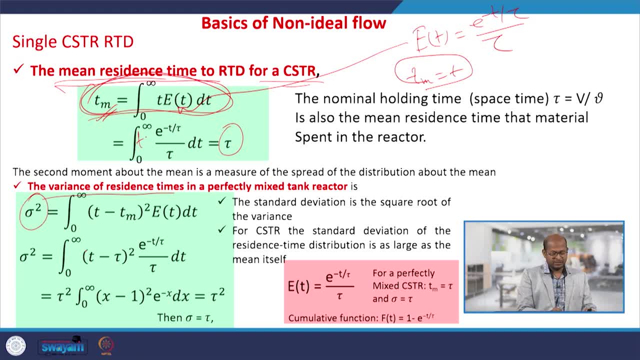 of the residence times for a perfectly mixed reactor. sigma square. the definition is this: Here Et we can substitute it here, This Et we can substitute here and after substituiting, if we do integrations. so then sigma square equals to tau square that we get. 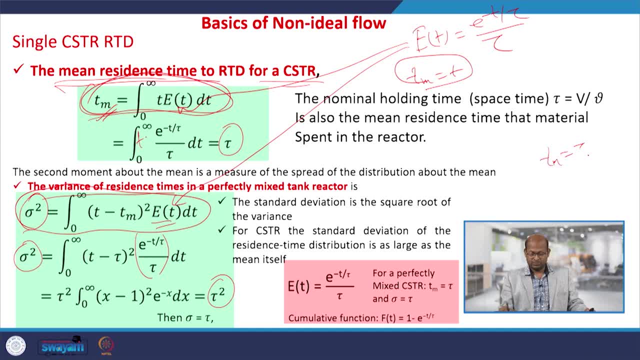 So sigma Tm equals to tau and sigma square equals to tau square. So this way you can write: or sigma equals to tau. So for a perfectly mixed CSTR reactor, mean time equals to tau and sigma equals to tau and Ft equals to this, Et equals to this. This way for a CSTR reactor, 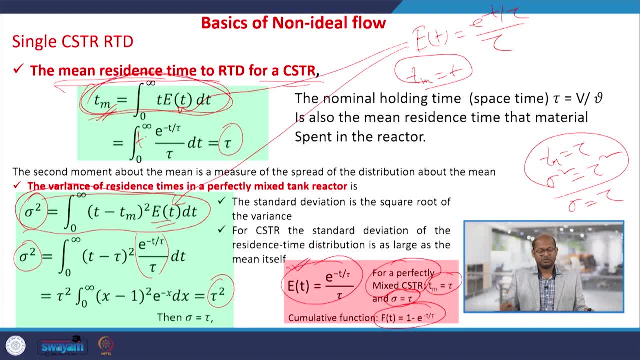 we can summarize that residence time distribution functions. Et for a CSTR reactor is e to the power minus T by tau. by tau, This is residence time distribution functions and mean time equals to space time and variance sigma equals to tau and Ft equals to 1 minus e to the power. 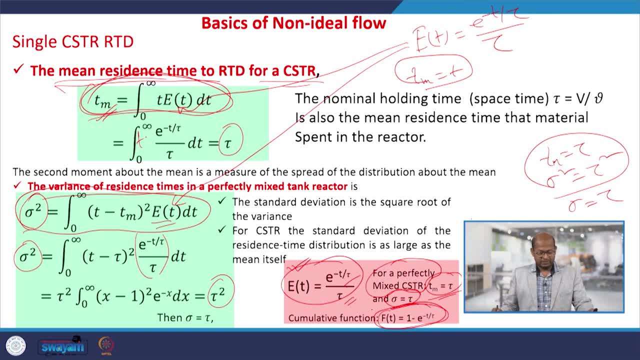 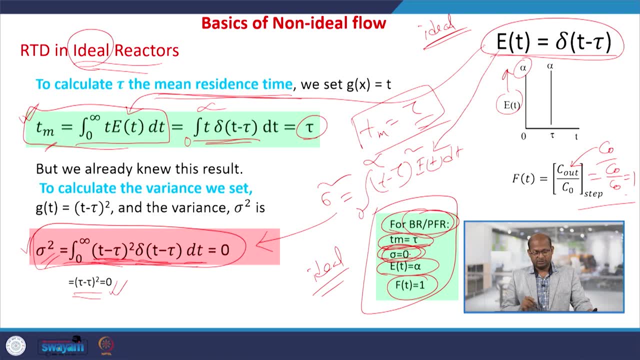 minus T by tau. So here, batch reactors and plug flow reactors, Tm equals to tau, if it is ideal. So sigma equals to 0, Et equals to infinite Ft equals to 1.. This is for batch reactor and CSTR reactors: Ft equals to 1, Et equals to infinite, sigma equals to 0, Tm equals. 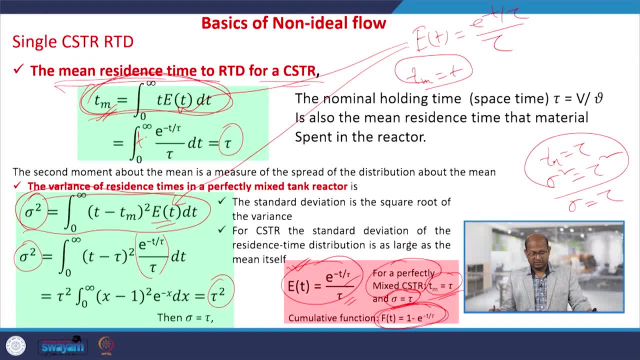 to tau, And for CSTR reactors Tm equals to tau. that is the common in both the cases, and here sigma equals to tau. There sigma was 0 and here sigma equals to tau. So this is the common. Here Et equals to e, to the power minus T by tau, by tau and in that case of batch reactors.